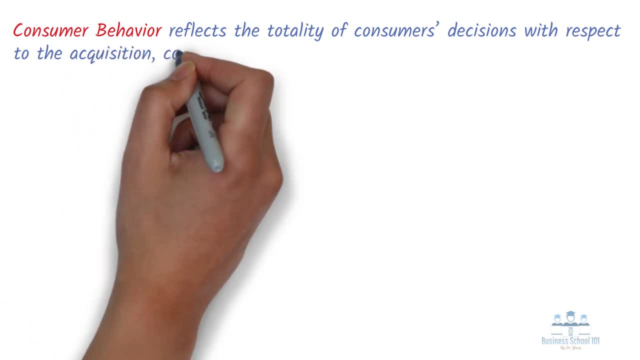 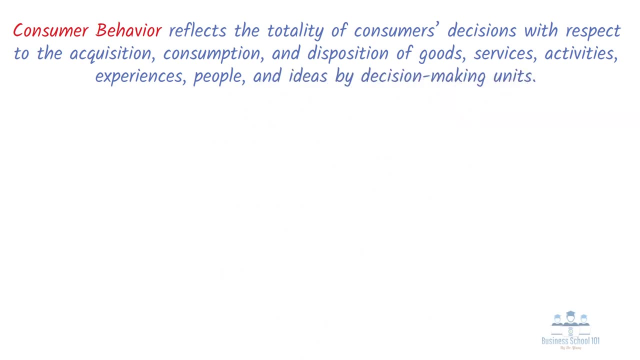 of consumers' decisions with respect to the acquisition, consumption and disposition of goods, services, activities, experiences, people and ideas by decision-making units. Consumer behavior includes not only buying tangible products such as books or cereal, but also includes the use of consumers' services. 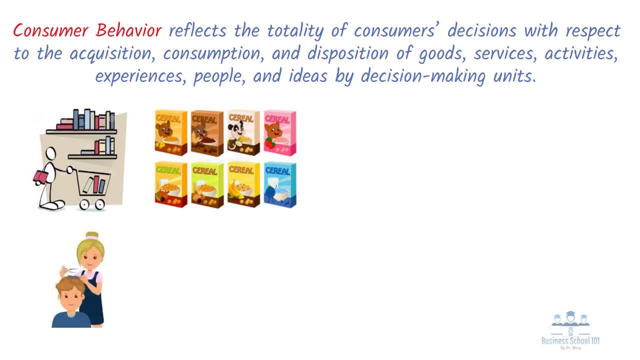 activities and decisions. Consumer behavior is a way of buying tangible products, such as books, and activities and experiences such as getting haircuts, going to a movie theater, taking a vacation and donating products at Goodwill. Moreover, consumers make decisions to vote. 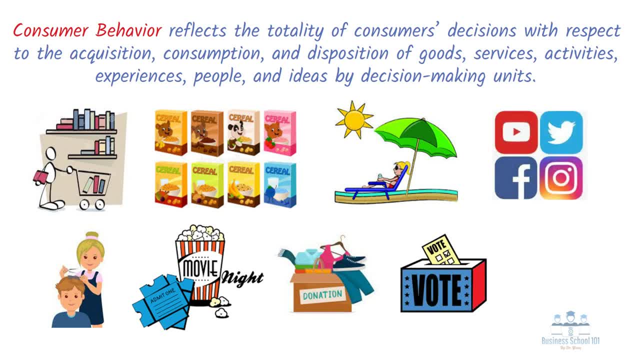 for politicians make choices to spend time either on Instagram or YouTube or decide to work out at the gym. Consumer behavior involves more than buying. There are three broad categories in which consumers make decisions, and those are acquisition, consumption and disposition. 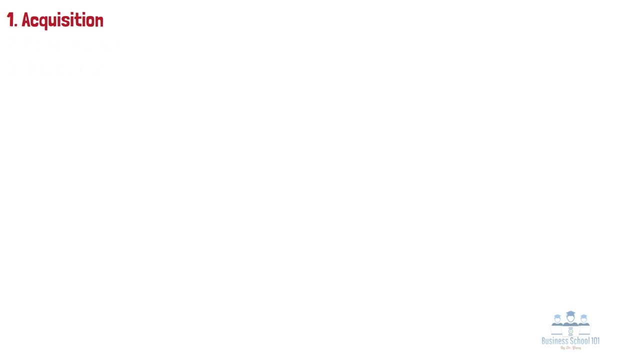 First, acquisition. The acquisition is a way of buying goods, services and decisions. Acquisition includes various ways of obtaining offerings, such as renting, leasing, trading and sharing. For example, consumers will compare the price of rental cars in different stores, such 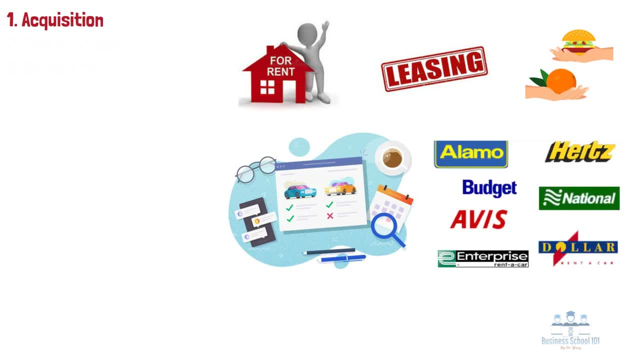 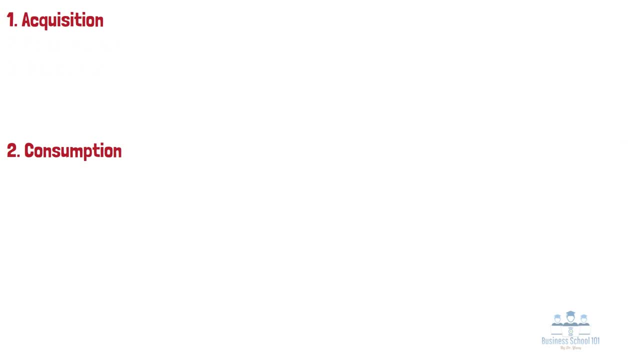 as Enterprise, Budget Car Rental or Avis, etc. and then they will rent a car that meets their criteria. Second, consumption: After consumers obtain an offering, they use it. Through usage, consumers can be satisfied or feel regret from the purchase, Depending on their experiences with. 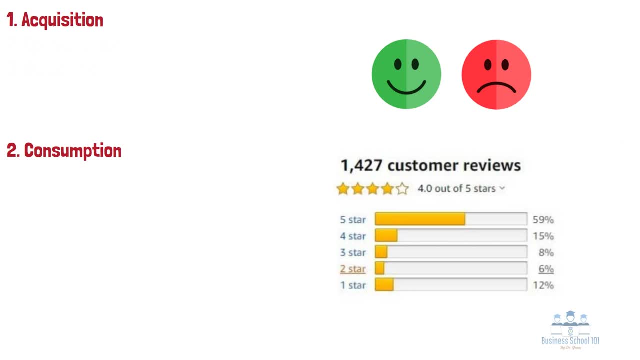 the usage, consumers provide positive feedback. Second, consumption: After consumers obtain an offer, consumers can make positive or negative reviews about the product or services. As consumer reviews influence other consumers significantly, it is important to satisfy consumers' needs and wants. Lastly, disposition: Consumers get rid of an offering in various ways and it also provides 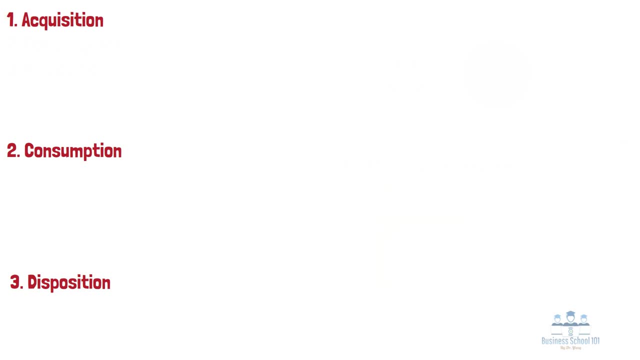 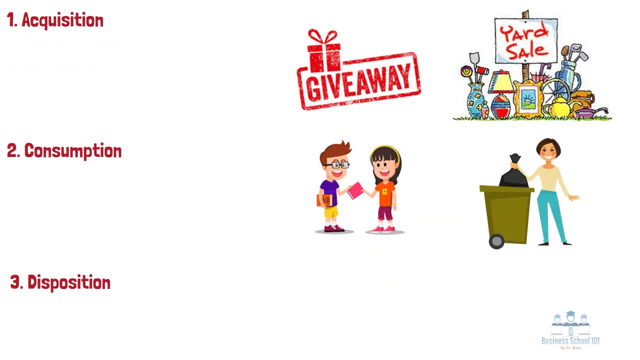 important implications for marketers. Consumers can give away their used products or sell them, lend them to others or throw them away. Environmentally conscious consumers put effort into recycling and or reducing waste, and they even try to choose biodegradable products. Consumers can give away their used products or sell them, lend them to others or throw them away. 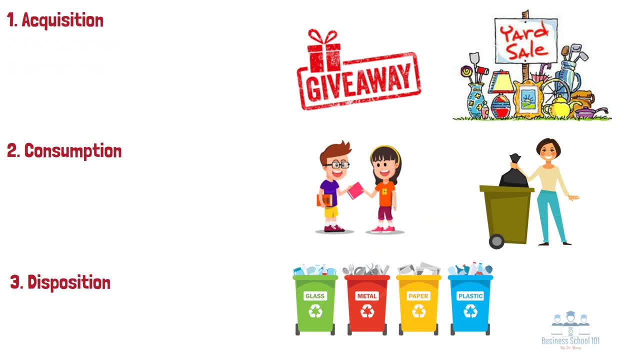 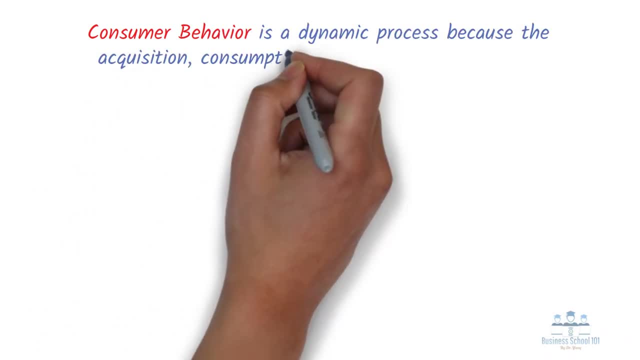 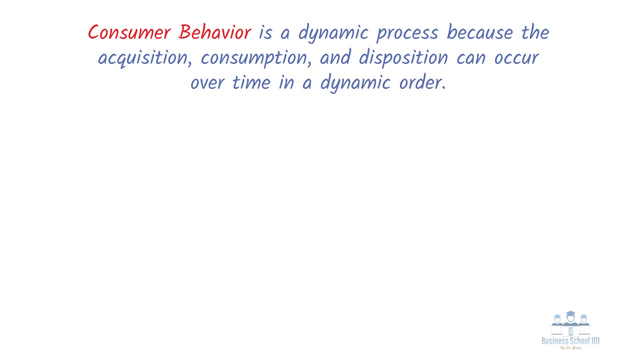 Besides the above three categories, please also keep in mind that consumer behavior is a dynamic process because the acquisition, consumption and disposition can occur over time in a dynamic order. It can involve many people in many decisions, such as where, when and how to buy a.